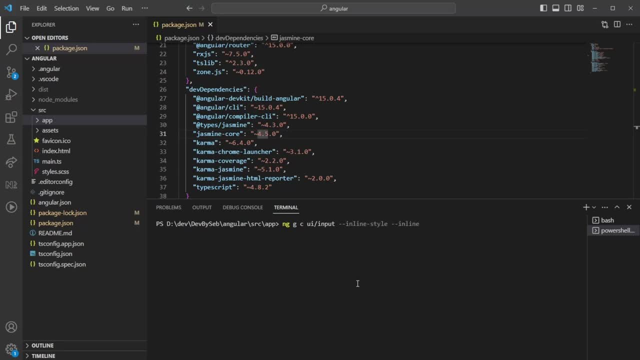 the styles, because we we don't want different files just for this purpose, and we're going to make sure that it's standalone as well, which means it doesn't need to be combined or added into the app module whatsoever. It will be complete standalone from the application. So, going to the input file now, 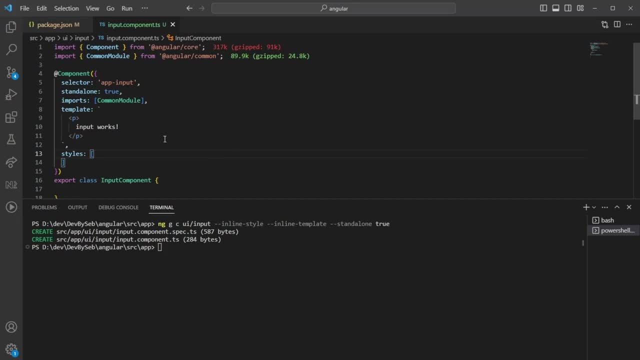 we have inlined the template, we have inlined the CSS here, so we don't need any other boilerplate code. So the thing we can do, essentially, we can go ahead and add- sorry, we can go ahead and add a div for a form control. We're going to add a label, also going to add an input here, So just 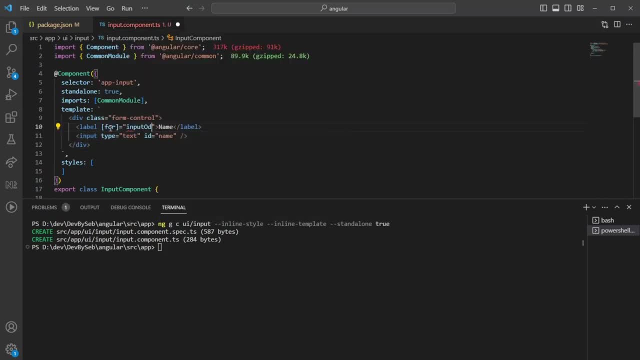 to make it more reusable. we're going to add an input id here so that it can be reused. We're also going to say it's, it will be the id of the input id here. We're going to prime the label, of course, and then we are. 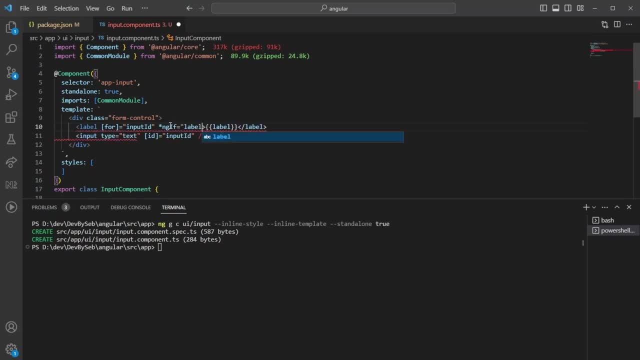 going to say: if we have a label we want you to print is otherwise we do not want you to print a label And we're also going to take in a value here. So now you can see there's a couple of red stuff. we need to make sure we have input, inputs for this, and let's go ahead and just close this. 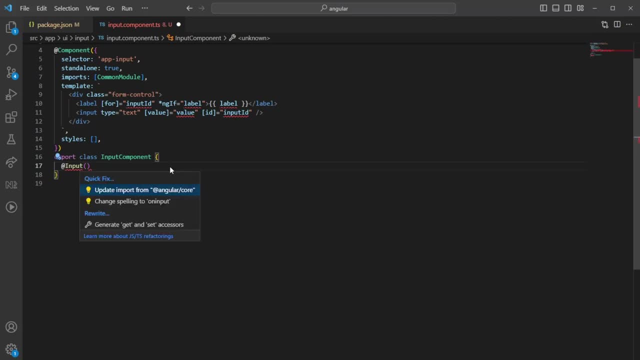 one down real quick. So we'll have an input, we'll import it, we'll say, all right, input id. we're going to to generate a random string. so just for the id, in case we forget to pass it in. If we do pass it in, it might be. 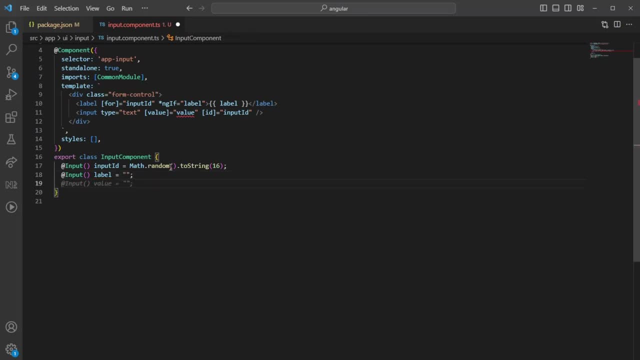 because we want to have automated test or something like this. but for now we're not going to to go that road också. we're going to have a value, but also we want to make sure that the type is something we can customize from outside. So we're going to. 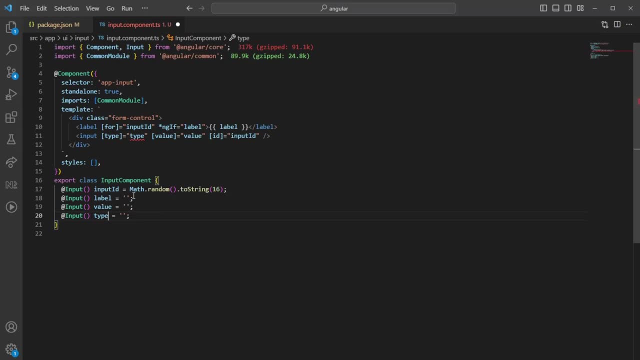 also want to add some type, all right. so what we want to do now, essentially, we want to say all of the values we pass in should only have a certain type, so we can say interface, sorry, type, input value in this case, and it's going to be able. 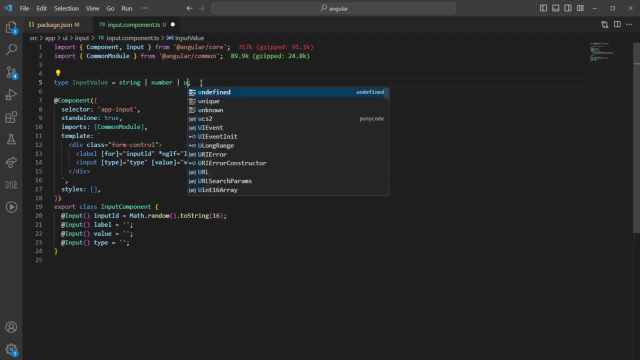 to take a string number and undefined. that's all. it's not supposed. you're not 100 sure that you're going to pass something in. it's going to be like this in this case. as for the type, there's a couple of things we want to support. so input type: 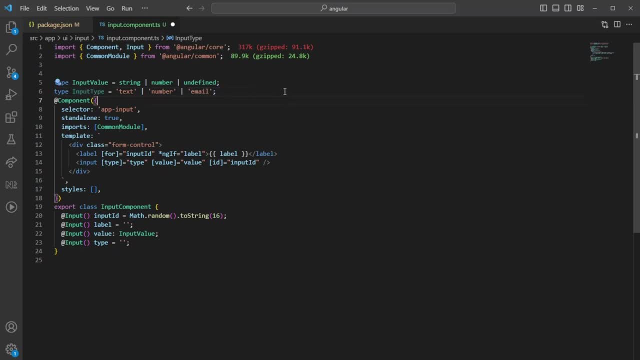 text number. email password is not needed for this example here, and you can go ahead and add whatever you would like. so the reason to why we have this is essentially, when you utilize it in the html, you can receive the error prompt immediately. there's no need to have enums, because if you have enums, you 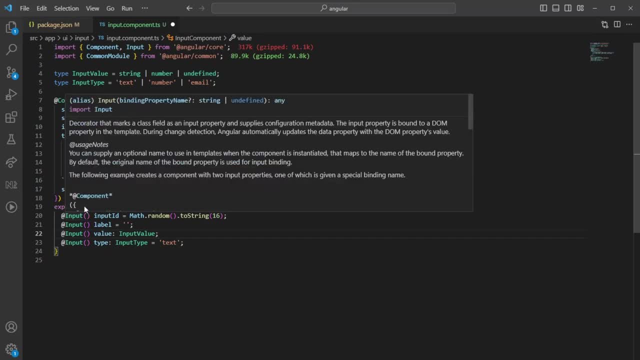 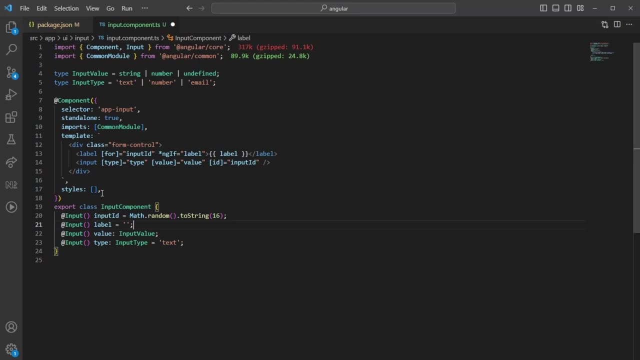 would have to declare read only prop in the component you're using it in order for you to actually utilize it within the html. that's why we're using types here. that's why i prefer to use types anyway. so once we're up here, we have the component, we have a label, we have an input. now 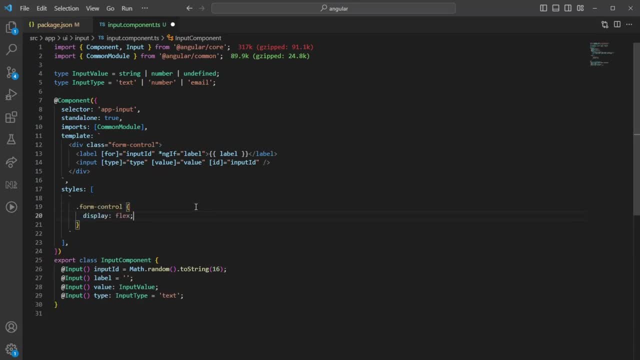 let's add some stylings for it to look a bit nice. we can say: for the form control, we want it to be display block margin bottom. we want to say 16px. forget about rems for now. we also want to say the label and the input once we want it to be appearing on its. 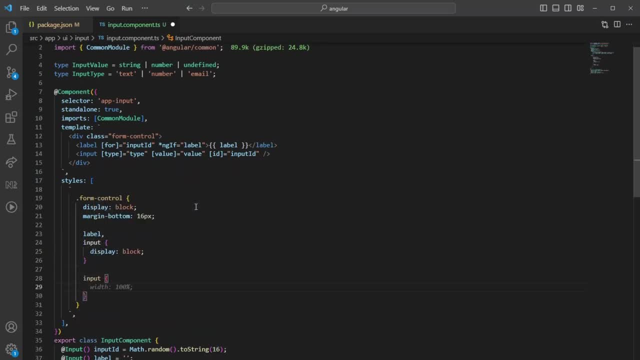 its own row, so we can say display block, and we want the input to have, uh, we want it to have a certain padding, so eight pixels in this case. border sizing, uh sorry. box border, oh my god. book sizing, border, box, sorry. and this is because we want the 100. 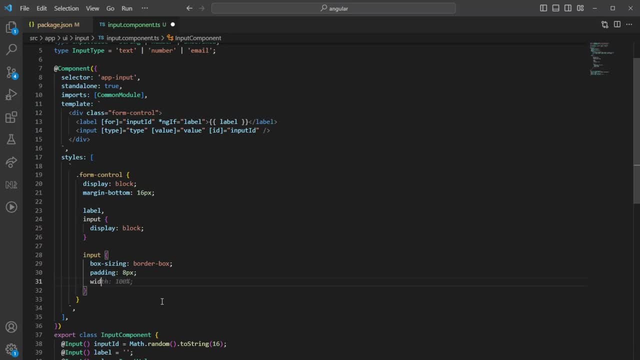 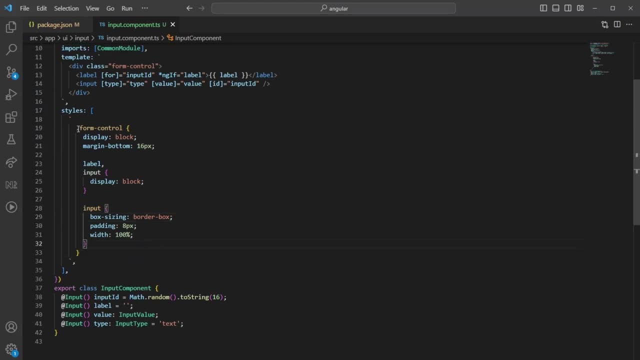 width to actually involve the padding that we have here, so with 100. so now we have a couple of stylings for it, so it looks not totally trash. it won't look good because it's- yeah, it's too little for now. we're doing this for the visual. 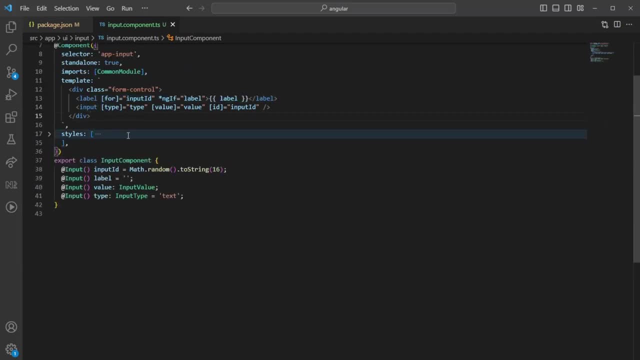 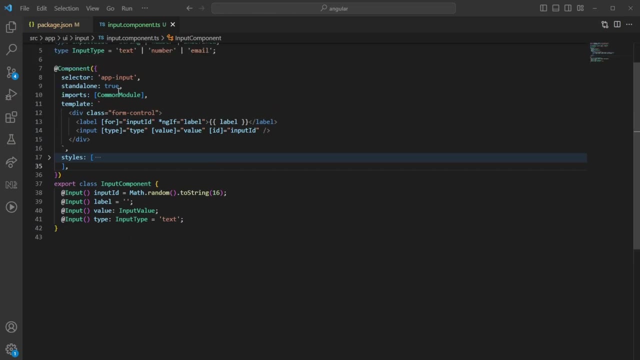 purposes. so we have styles, we have html for it, and now what we can do is, essentially, we need to make sure that we can export it, and we're getting to that part shortly. so it's defined to be standalone, hence we need to import a common module in order. 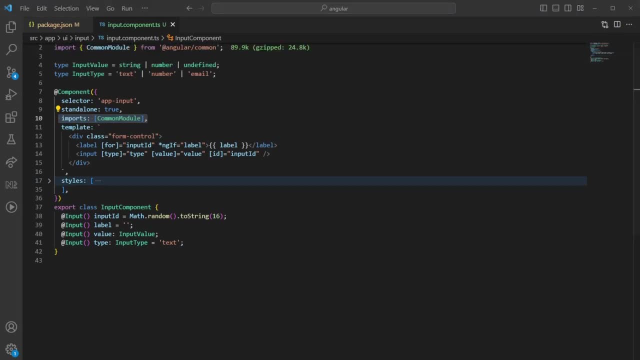 for use to utilize angular stuff. that's specific for the application. so what we can do now is there's a couple of things we want to do, so we need to navigate to the main ts file and this is the way you would bootstrap a normal angular application. 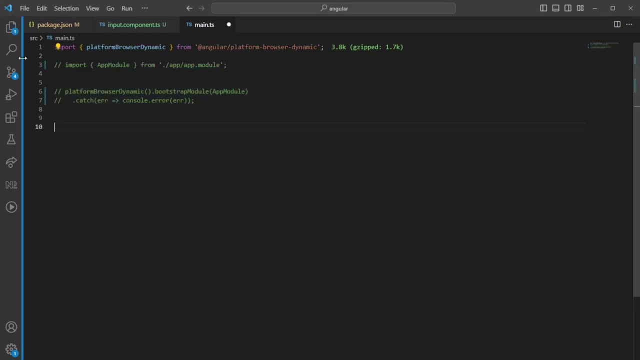 and hence this is not a normal angular application. so we'll just comment this out real quick. we're going to add an async query function like this. so here we're going to generate the app, so we're using it so that we can use that weight here. so we'll create an application. 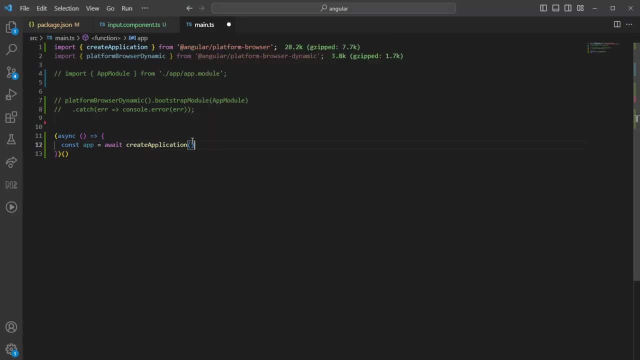 through the angular browser that we're we're utilizing here- platform browser, and here we're going to specify the providers we want. in this case, we have no global provider, so just skip that for now and we're going to say, hey, we have the input element we're going to generate, so create. 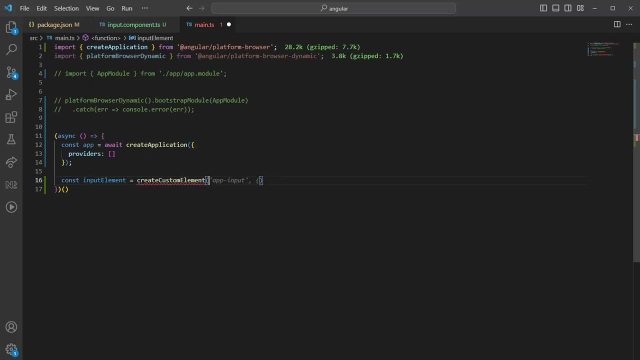 custom element. and here we are, in, in, let's see here, let's import this. it should be coming from: yeah, custom create custom element should come from. import custom element from angular elements in this case. all right, so once this is done, hovering, we can see the first one is going to. 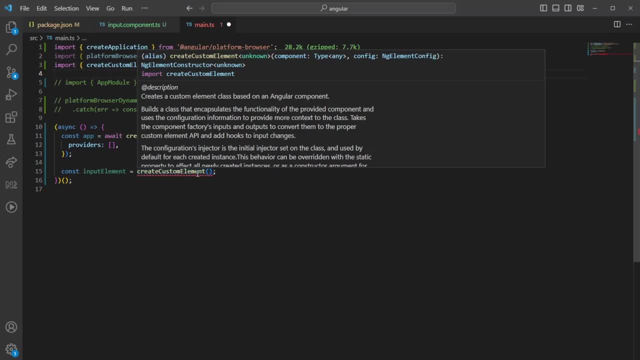 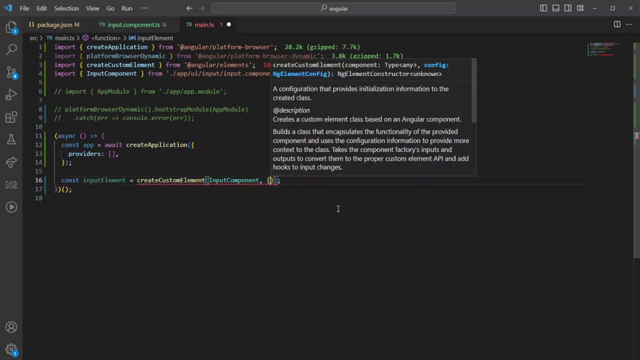 become component. the second thing is going to be the, the actual element, so, or essentially, the config of the element. so first, here we created the input component and in for the second one, it's going to take an injector. that's all that's mandatory in this case, and we're going to fetch the injector. 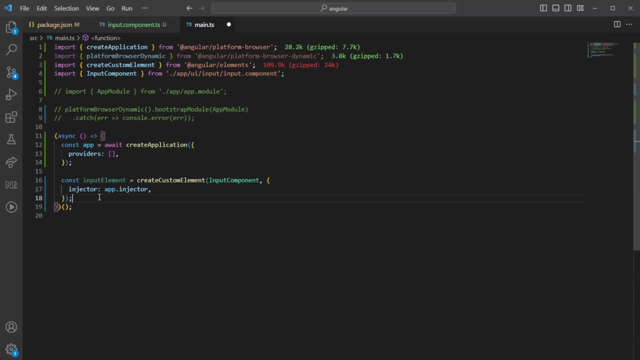 from the app that we created. so now we have essentially created a custom element, but we also need to define the name of it. so in this case we're going to go with custom elements, dot define. here's the name we'll actually make sure that it gets when we use it in the other application. 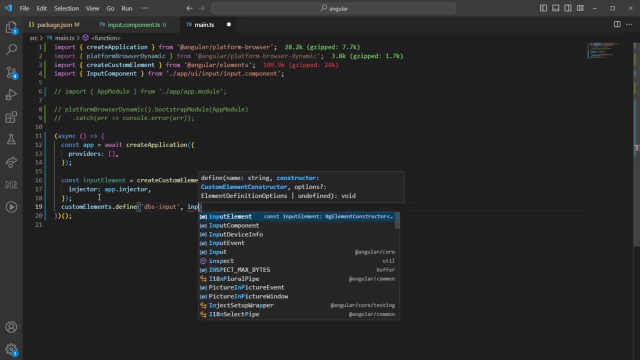 i'm going with dbs for dev bicep input and we're going to pass in the input element here. so we're saying, ah, you're going to use these tags, so in this case, in the other application, you would utilize it in like in this way. so hence this needs to match. it's the selector that you'll. 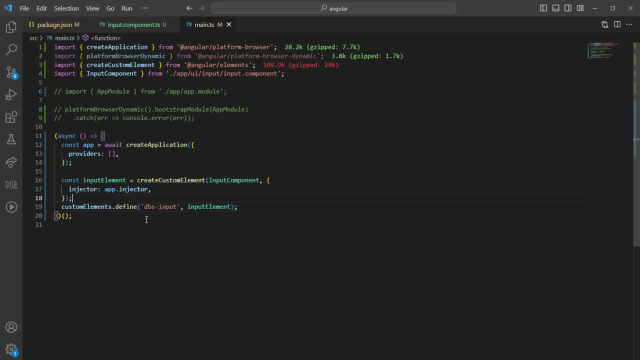 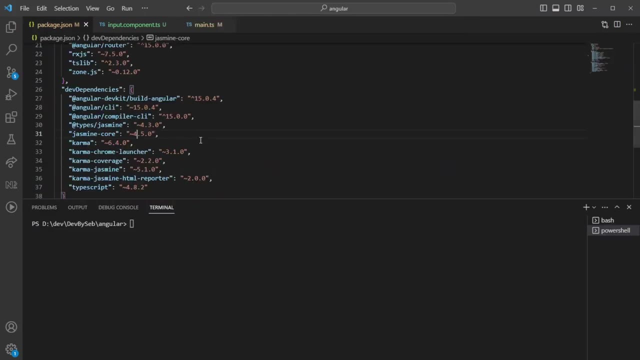 essentially have when you use it. so now, when we have something like this, we should be able to build it and use it within an html immediately. so what we can do in this case, i'm going to create an output to build. this is actually what you see on the screen right now. 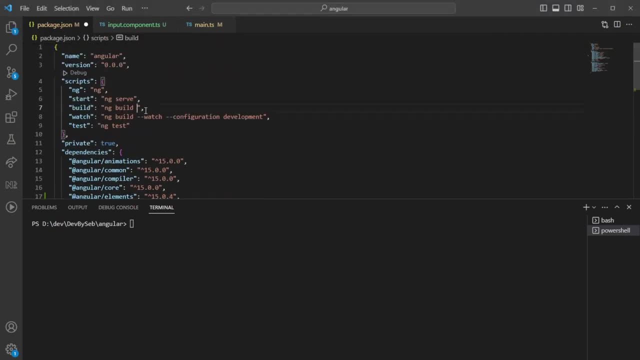 so we're going to do this and also let's navigate to package asian before real quick. there's a couple of things we want to do, all right. so for the build we want to say output hashing none. the reason to why we want this is essentially we want to remove the hashes from. 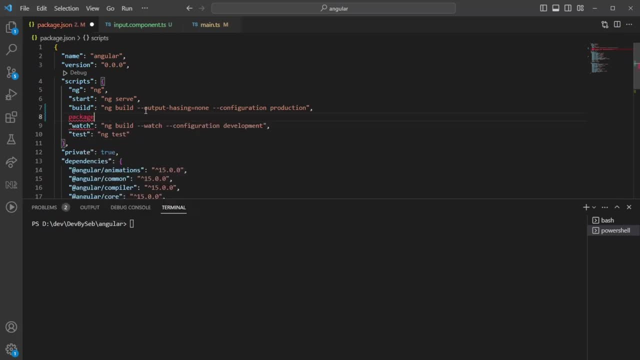 the build, because we want to combine the files that we're building into one file, so, and we also want to package this application so that it appears within one file so that we can easily copy and paste it, right. so this we're going to essentially here to essentially combine runtime polyfill, polyfills main, and we are going to- yeah, we're. 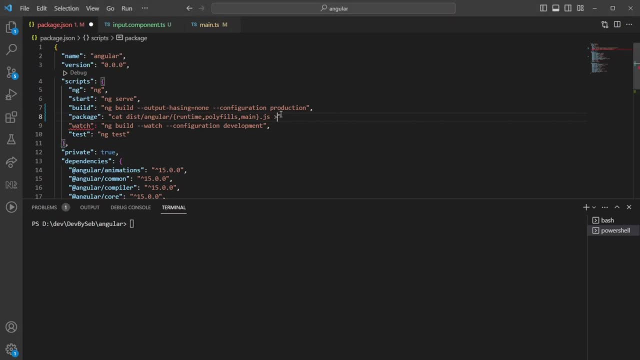 going to send this into a specific, specific file that we have. so in this case, this angular component, let's call it component libjs. so in this case, when we build it, we'll receive a couple of build files. we can go ahead and try this out and you'll see what happens. so when we build the 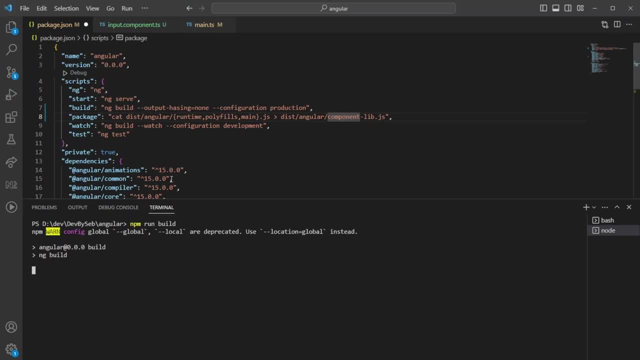 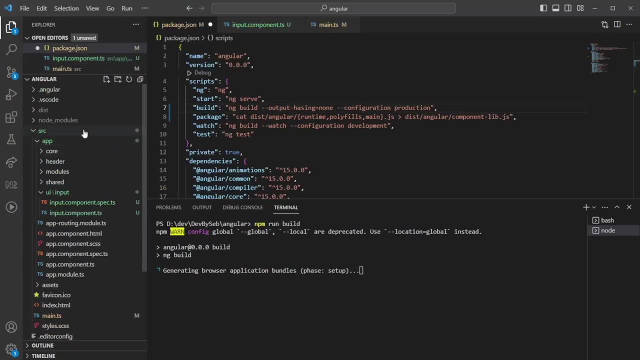 project now, given we don't have any errors within the application now. also note that it's not running with output hashing and so on, and you will see why and you will see what's happening. so it will generate this folder here with a couple of build files. so allow it a couple of seconds. 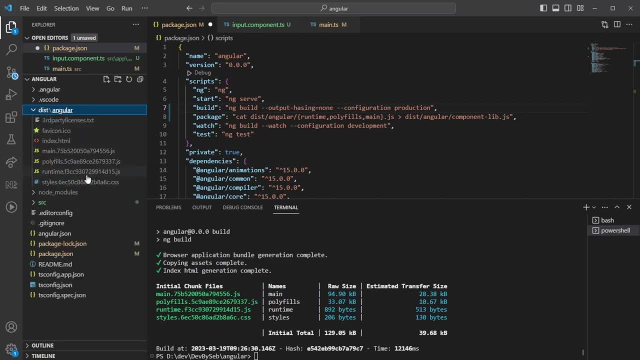 so you'll see here it has a lot of hashes here, so it will be extremely difficult for us to actually select these files. so output output hashing in this way will will remove all of the numbers, so it will be only main polyfill and runtime and this is what we're going to use to combine into the next file that we have. 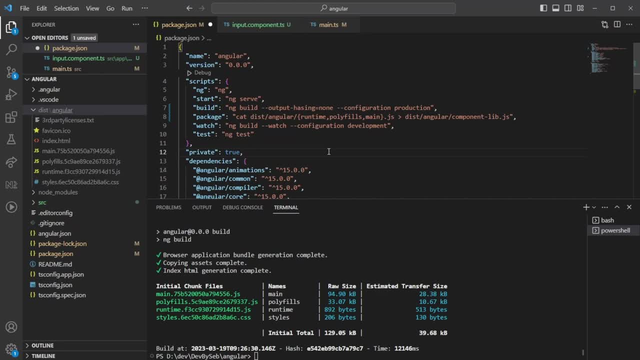 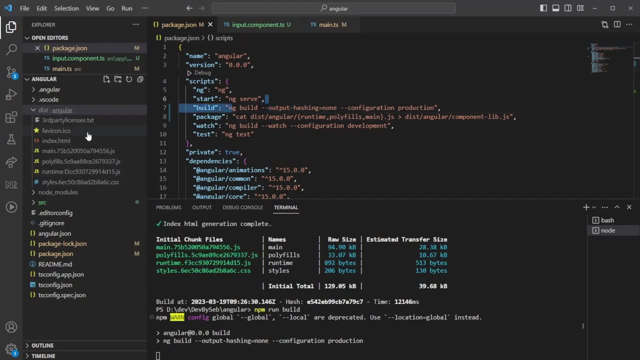 all right. so once this is done, uh, let's see here we, we save it, so we need to rebuild it now with the correct build options here, so it should be output hashing. so, building it again, it will run this with output hashing and you'll see the difference here within the naming of the files. 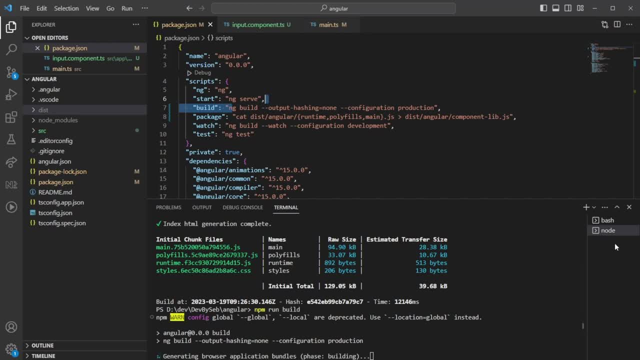 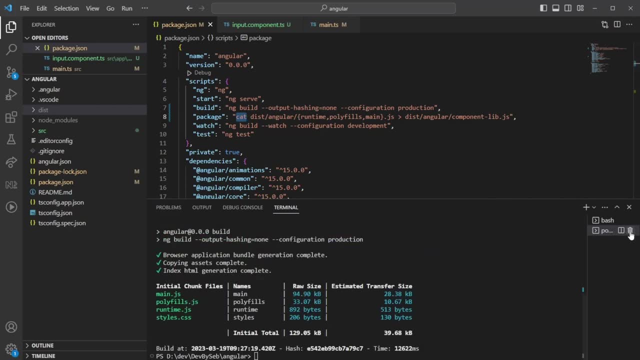 so allow it a couple of seconds and, since i'm using the catter, keep in mind that this is something you can utilize within bash. it's not something you can utilize with the powershell. so i would just close this and utilize my bash. i think the equivalent of it would in windows would be type, but i'm not entirely sure you can. 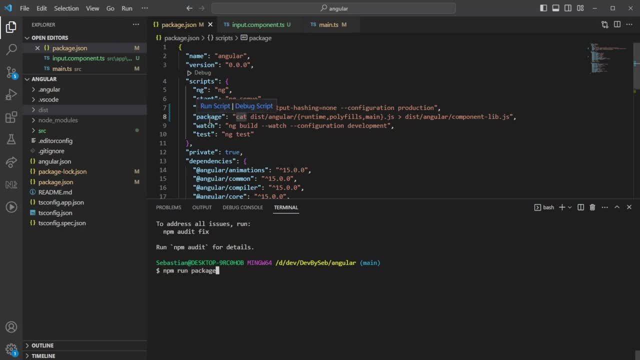 look that up real quick. but anyway, if i run npm run package now, what should happen here is that it should combine these three files into a file name component lip. so now we have this file component, which essentially is a mix of runtime, polyfill and main, and this is something we can utilize within our 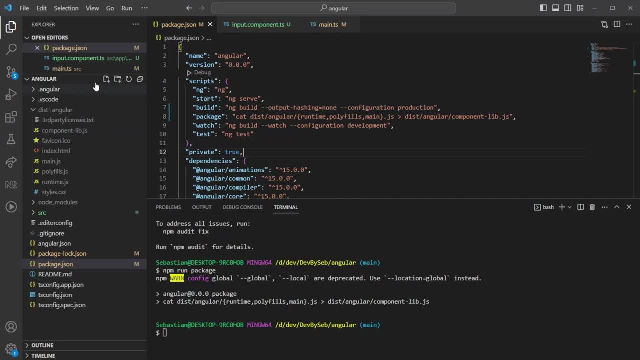 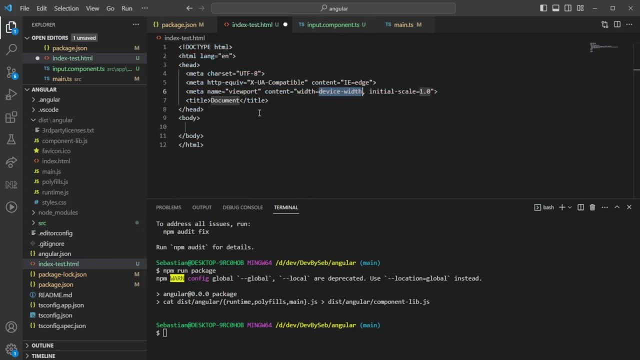 new html application so we can just copy this script file and utilize it wherever we want it. so we'll go ahead and just add a index test hdml file here. we'll give it a couple of html file features. we're going to import a script here, so since we're in the in the same folder, we can go. 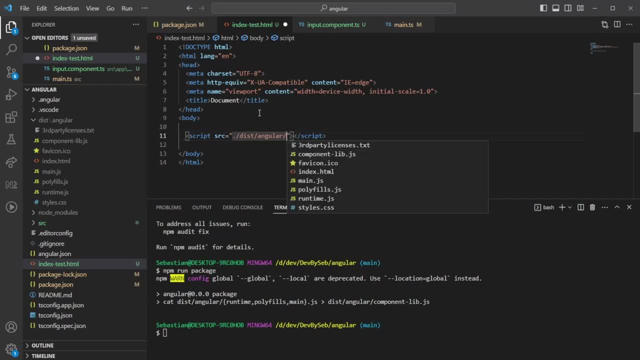 and then say: in the this folder, in the angular folder, we are going to select the component lib. here and now, within this html document, we can start using our dev bicep input component that we generated. also, we can pass in a label, my label. we can pass in a type. this is going to be text. 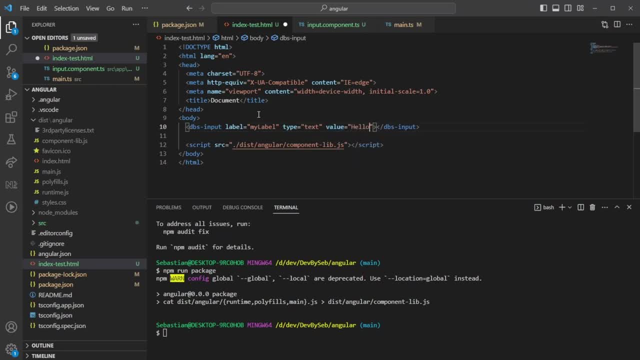 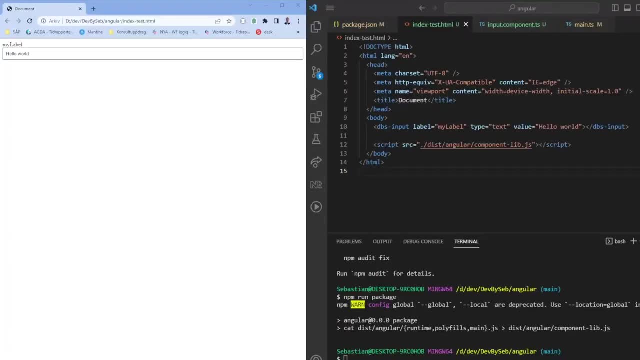 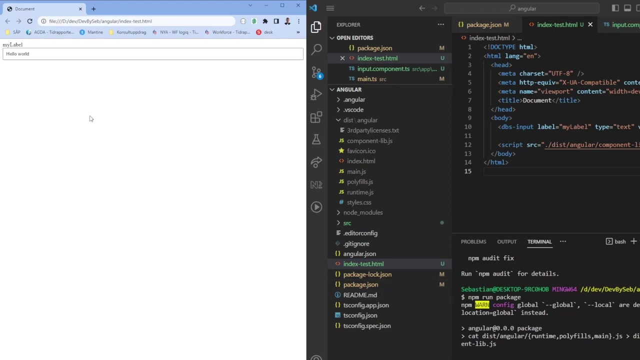 we can give it a default value here, which could be hello world. so, saving this and opening, i will open it in a browser real quick. all right, now, that's we're that. we're back with it. i just essentially opened this index tx file within the browser here and we can see that it in fact has. 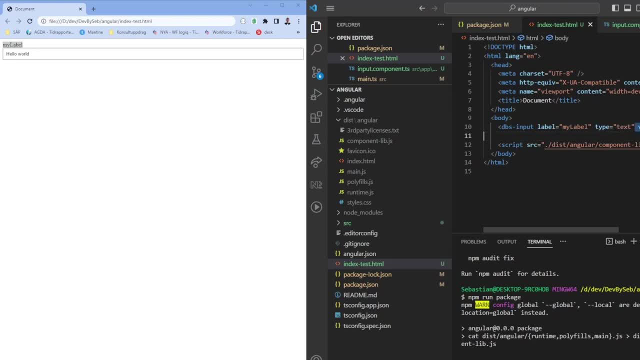 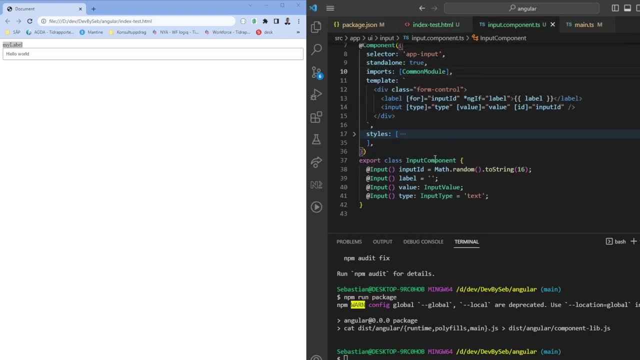 a label, my label. it also has the, the value here, which is essentially hello world. and you might now think: how can i use this within our html file? so, as you might have noticed, we didn't add an output listener, so we're going to go ahead and add an output here. so, once when value. 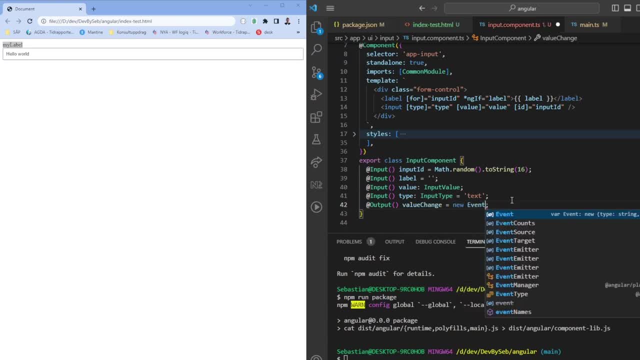 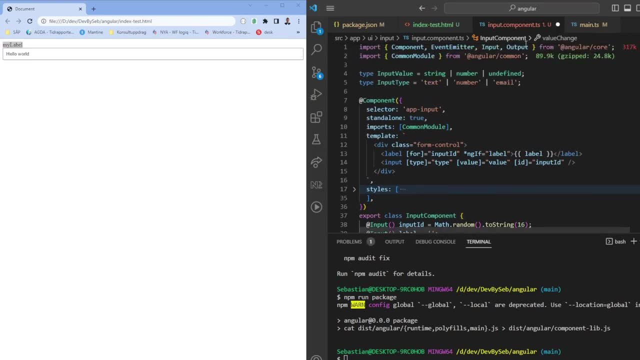 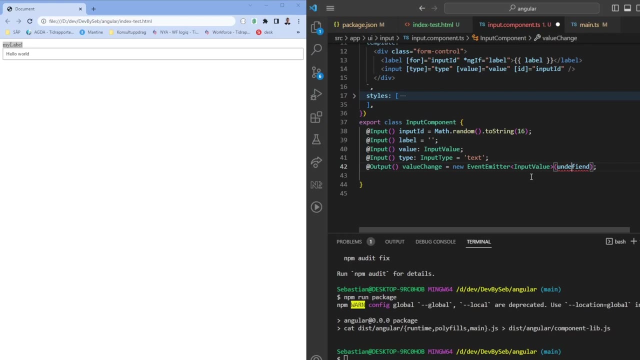 changes. we're going to emit the value so that we can set up a listener to listen for this within the html. this is just going to be. let's see, we imported it from angular core as well. perfect, so it's giving the input value here defined, all right, so when we change it. so on input, we're going to just say that. 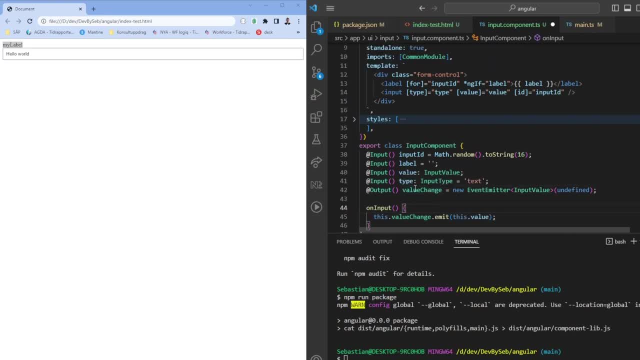 this value change emit, and we're going to set the value here, so we can add a lot of logic here, and then we can set up the listener, and hence this is the event listener that we need to set up from the the index test html file. we'll get to that shortly, so now the next step would 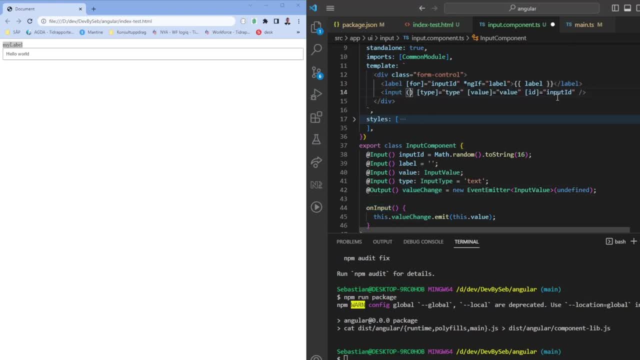 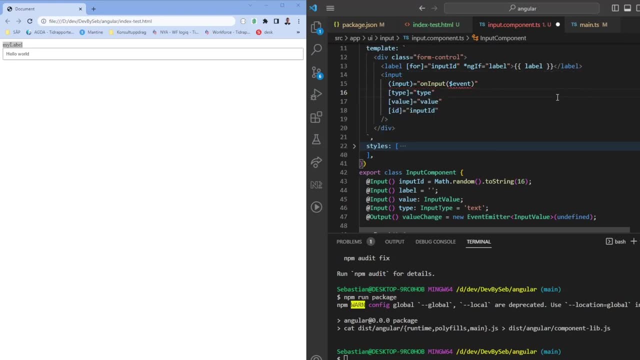 essentially to make sure that we have this on input function. so input, so this means whenever you type something, we're going to do this. and also keep in mind that we are going to pass the event here, so we need to receive it and we need to mutate it. it's here event and then we're going to. 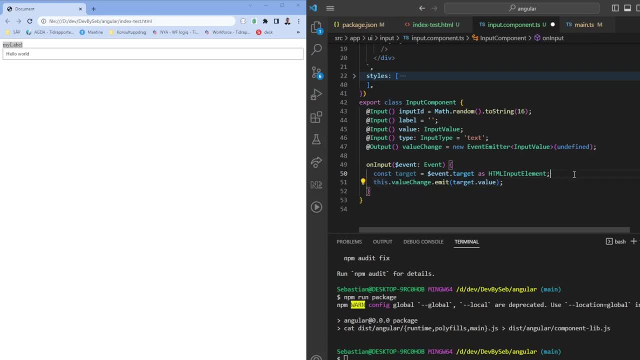 say that target and we're going to pass the event event. so we're going to do that and i'm going to pass in target value. so this value equals to target value, in case we want to have the the value still in this, this one, all right. so now we're pretty much set up for it. so 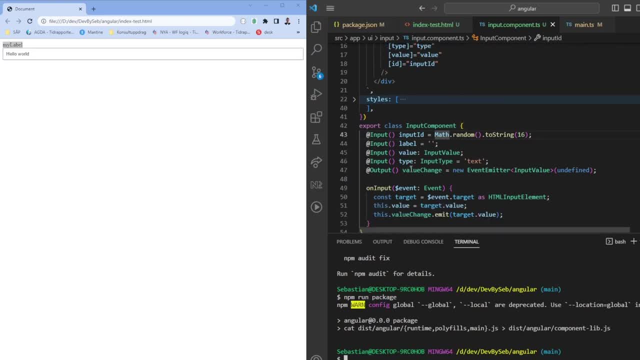 always remember that when, when you build or change something, you need to, you need to need to build and you need to repackage it right. so you need to run npm run build and npm run package. so what it does is it will create a build and from the build, it will package it. 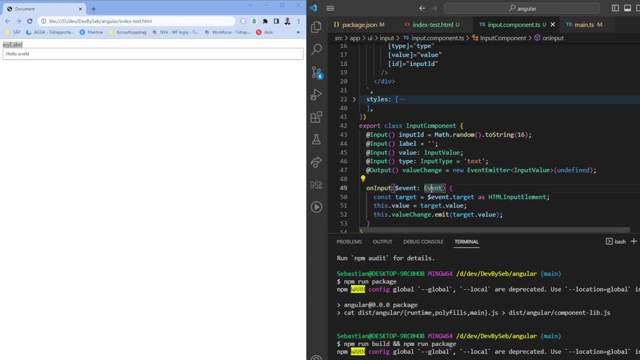 into this file that we have. so once this is done, we should now be able to essentially just start working with it, start creating the, the reusable components that we just generated, and so once this is up and running, now we'll see reloading. no change, but what you need to do here since this. 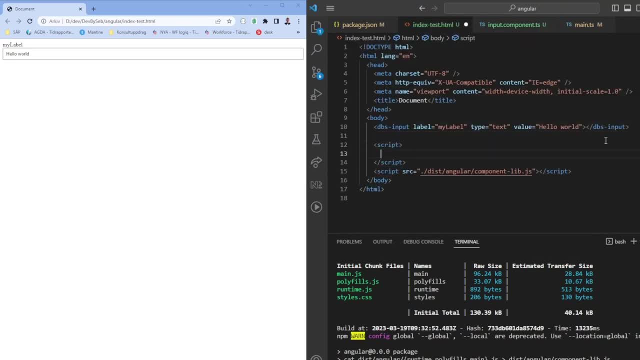 is html. we need to use the script here to bind a couple of things. so what we will do in this case is: let's say we have the label hello, or let's say name, and then we would have email. i would say email, and then we would have i don't know something. i'll say. 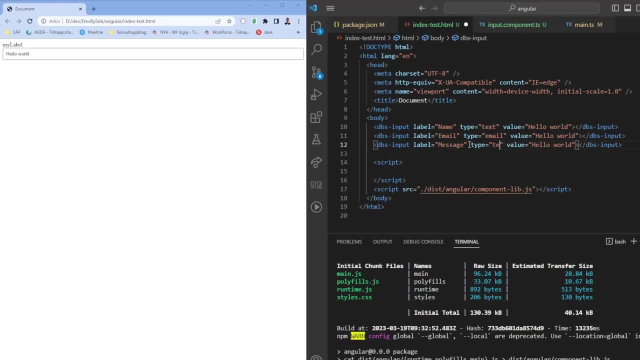 message. in this case i will have a text just for visibility. visibility purpose, all right. so reloading. we should see we should have a couple of things already here. this should be of type email, and now we should be able to wrap it within a form and we can add a button here. hence i'm adding it outside, so we don't have a, so it's not bound to the actual. 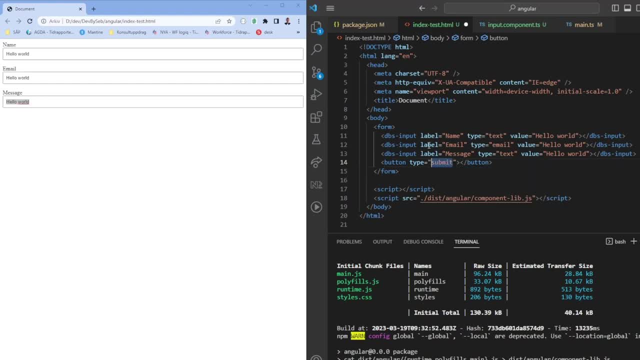 form. but we can move it inside. but we need to say this is going to be a button, so that it does not automatically submit the form when we press it. so when we press this button- sorry, i'm using angular logic- so when we do this we should get form values. so now we're going to essentially try to fetch the. 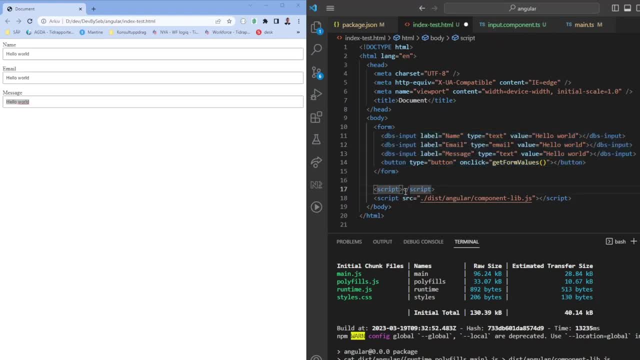 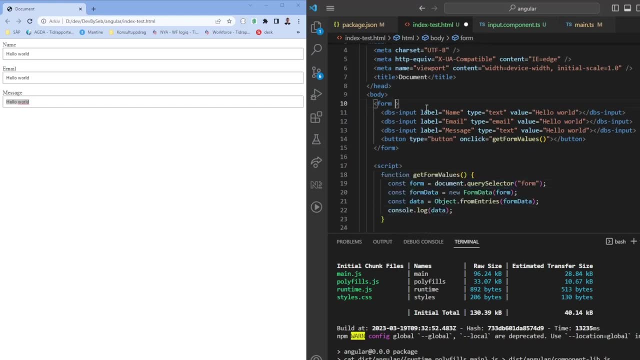 values of the form in this case. all right, so what we can do now is essentially just create a function which would select a form. so maybe it would be much better to get a user an id here instead of having the query selector. we can set get document a get element by id. sorry, 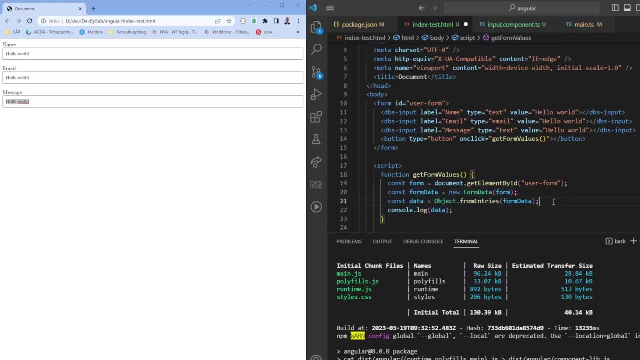 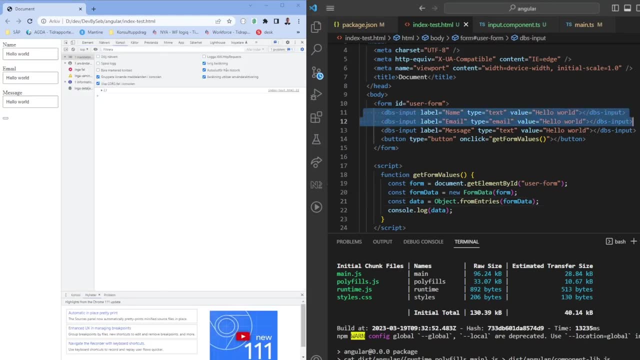 and we can fetch the form data and we can print the form data in this way. this is the normal way you would have to do it, but since this is essentially um, using our elements here, this won't work, unfortunately. so what you would have to do in this case is, essentially, you would have to fetch the form and then you would say: the form. 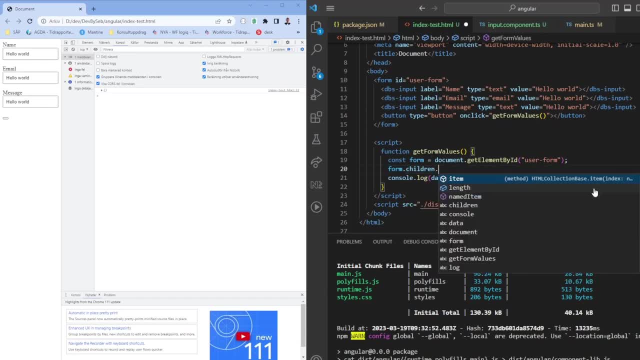 children, um, and then you would have to loop through it. so let's say we map in order for us to get an object out of this and we can say: cons, data equals to this: remove the array syntax from here. it was just a mistake, um, and here we're going to return the, the label and. 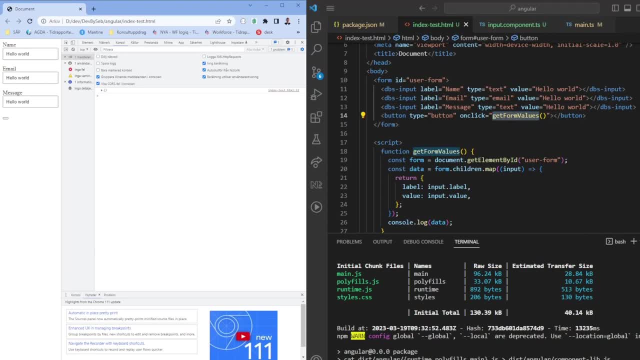 the value of the input for each field. so every time we press the button we should be able to get the values and all. yeah, sorry, we need to do this arrayfrom, generate an array from this. so now we should have an array and you can see we have undefined. 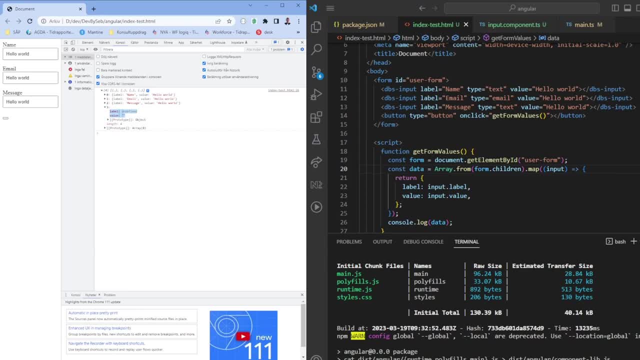 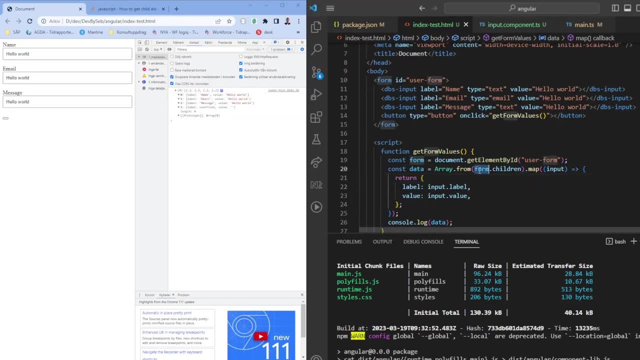 and value. this is the button that we have, so we need to make sure that we in some way can remove it. all right, so what we can do here- since it's not really, since it's fetching all of them- we can change from from children to query selector, all and here we can essentially say dbs input. so we're. 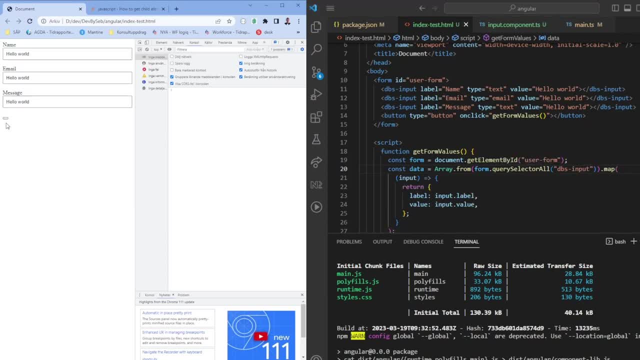 selecting them by our input. so if i reload and i click on the submit, in this case let's add the text, so submit or whatever we wanted to do, you'll see that we have the values. changing the message here should also change the value here. so with a simple function here again, you're not going to see. 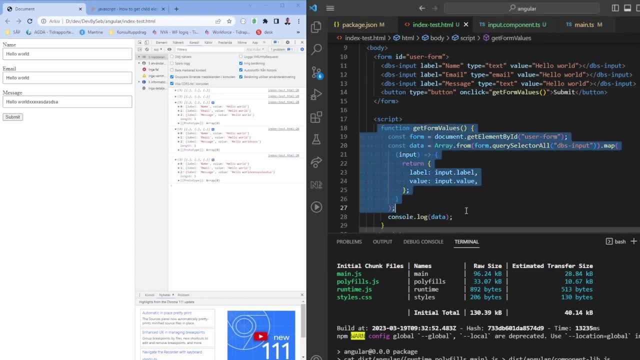 the背景 published. so we're not going to be using this event window here in the valve, but you can see that we have the values here so we can save our result here, and so let's see if we want to change the value here. you can see, we can see here. you can see that we have the values here, so we can. 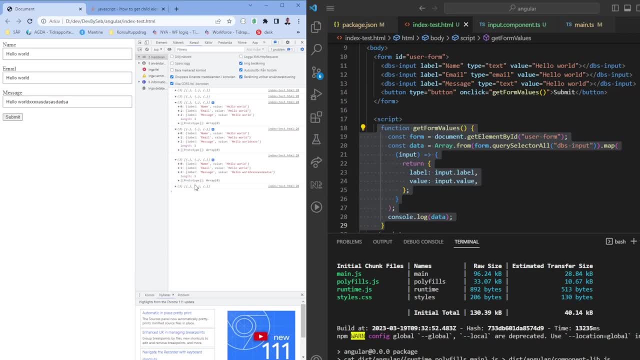 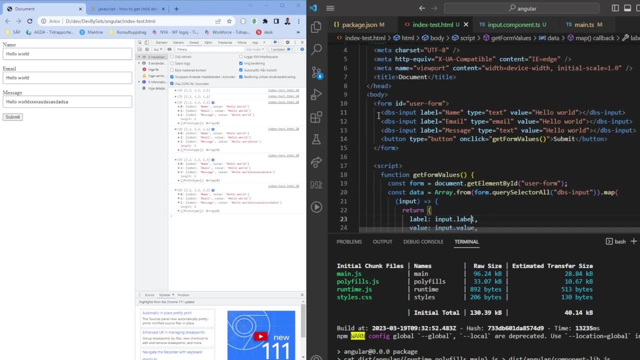 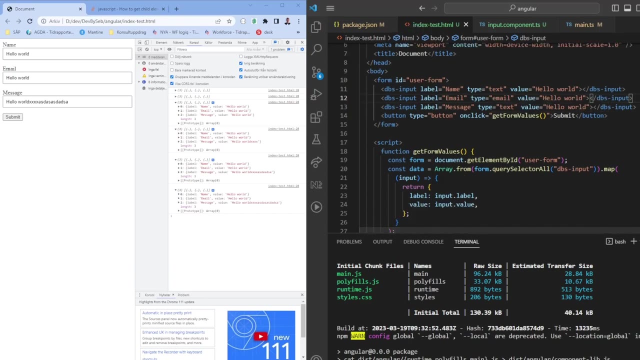 here, which we essentially could build in if we wanted to, and created a like custom logic for for this, to print all of the forms. this is one way of actually utilizing the angular components generated to angular elements, which, in this case, is used within a basic html file. so what? what can? 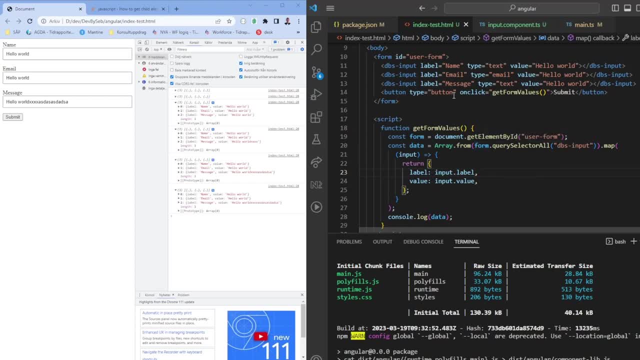 we do now in order for us to actually, let's say, we want to set up listeners on the value change that we had. so there's a couple of ways you can do this right. so either we could say array from and then from dbs input, we could say: for each one of the elements we are going to set up, a couple. 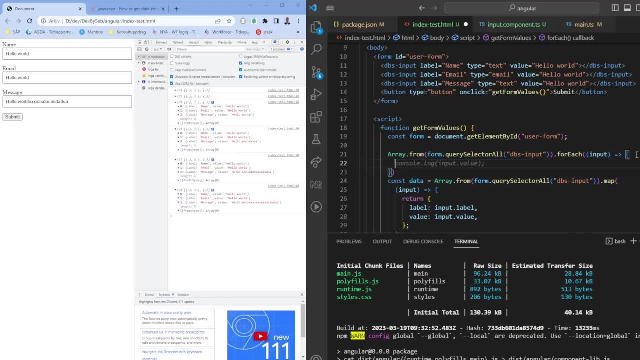 of things, so we can set up listener for all of them, if you would like to. i don't see any point, unless you are actually um add event listener. sorry, add event listener, and instead of inputter it should be value change, because this is essentially what we're outlining.